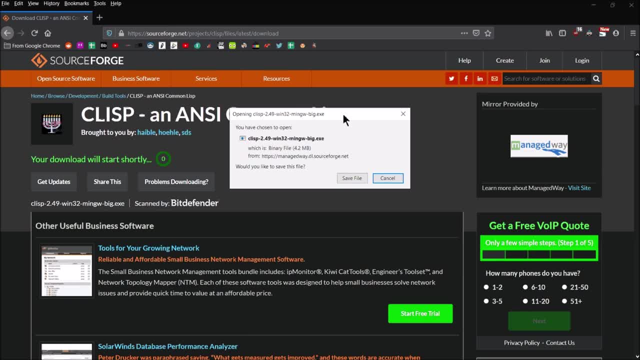 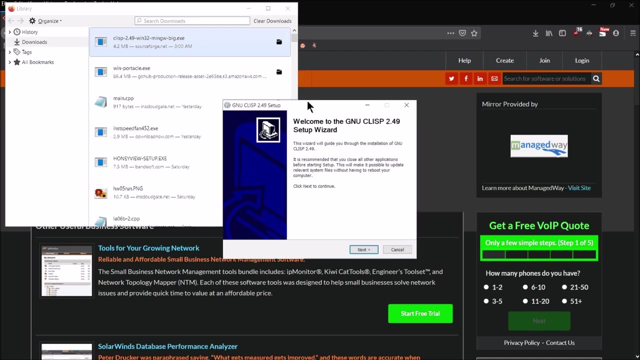 Right, and then the window will pop up. Go ahead and click save file. Save it to wherever you want. Save it to your machine. Once that download's finished, you can just double click and run it. Okay, you got your setup wizard. 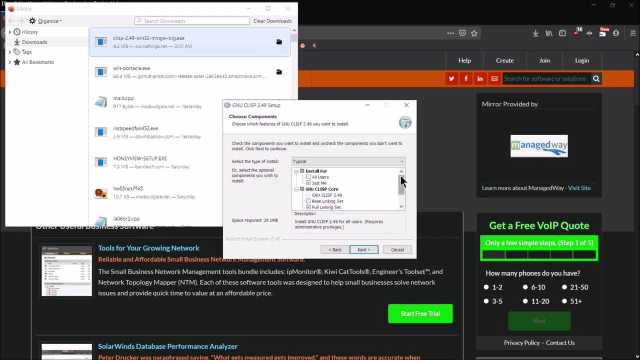 It's going to go by pretty quick, Right, and you can put this wherever you want. Typical is probably going to work just fine for you. I want to put this in a different location on my hard drive than the default. I'm going to put it on my F drive. 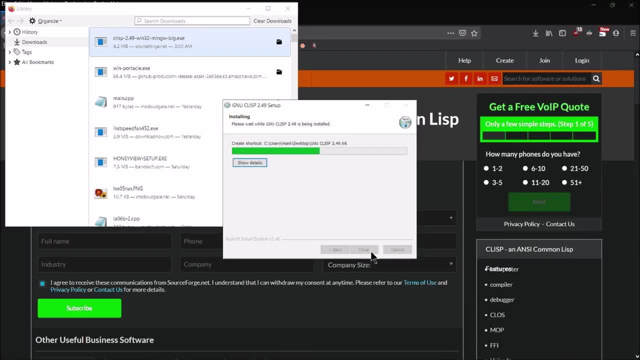 Fine, put it wherever you want. Go ahead and hit the install. You know it's going to do its thing. It's not going to take too long, Okay. And then, once it's complete, go ahead and hit your close And you're installed and ready to go. 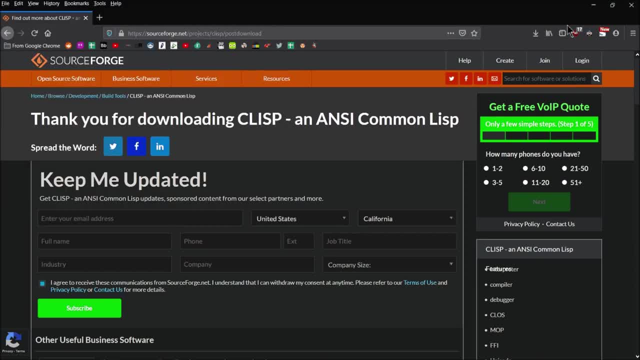 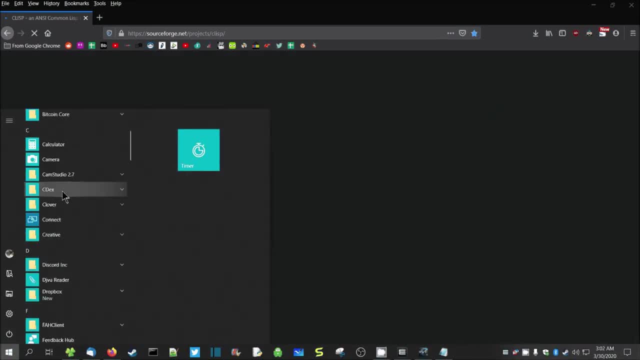 Then, when you're ready, you can go ahead and go to your start menu And then search for C LISP And then search for C LISP. Then, when you're ready, you can go ahead and go to your start menu And then search for C LISP. 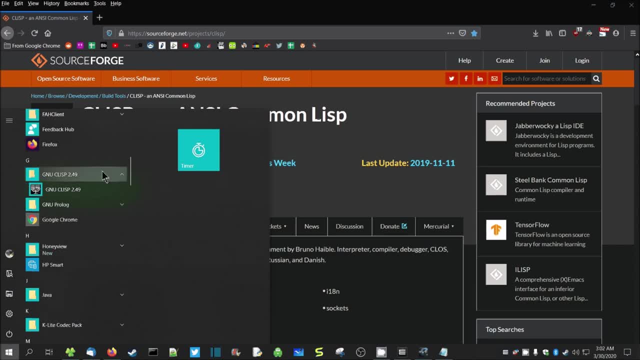 It's actually under a new C LISP. It's actually under a new C LISP, So you can go ahead and do that. You might want to right click and set that on your taskbar for easier access later, And then you can start it by clicking on it. 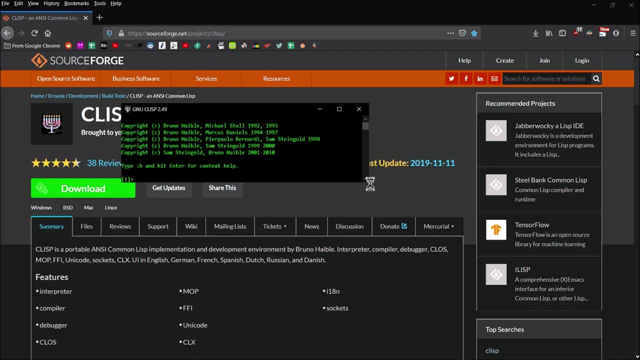 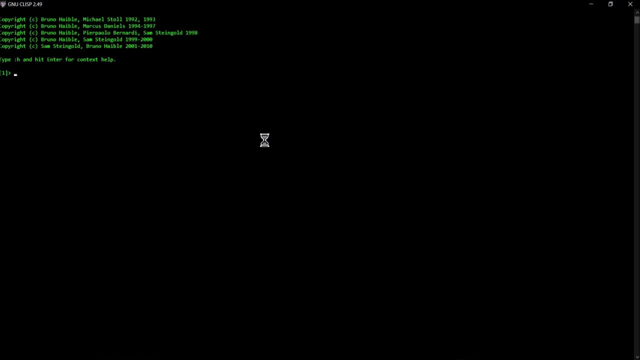 And then this brings up your interface. Okay, So this is one way that you can use this program, And From here, what you're presented with is a prompt where you can start typing in your LISP commands. So there's this high level interactive loop. 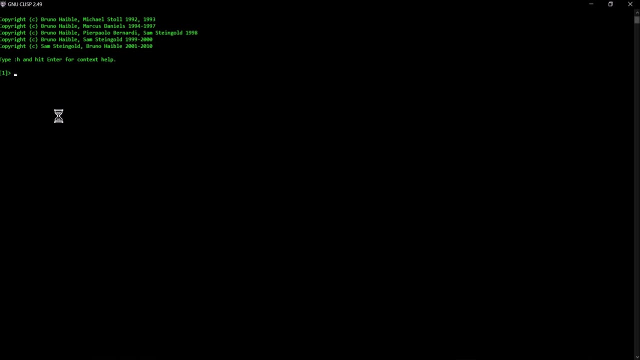 And generally the way this works is with LISP is you type in a command and then the interpreter in this mode will go ahead and process it for you. So if I wanted to print hello world on the screen, for example, I could print. 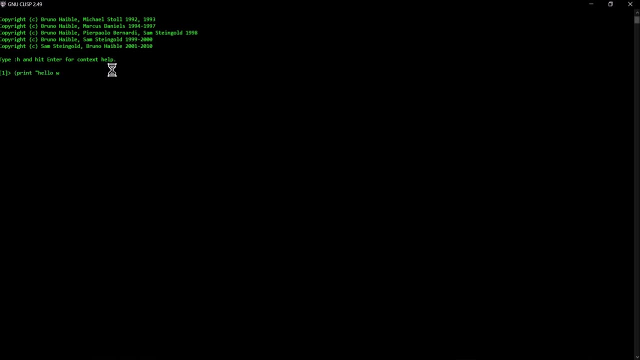 So if I wanted to print hello world on the screen, for example, I could print Hello world And you can see. there's the response from my command, right. So I made a call to the print function, passed it the argument. 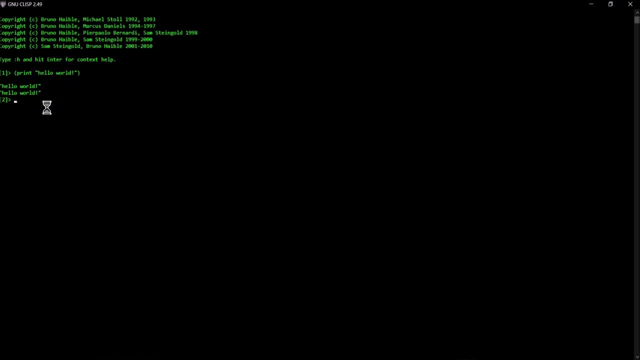 Hello world And I've got my output Okay. So if you want to get help, you can type colon H and that will give you some contextual help In this case, If I want to just quit, Since all I want to do is print hello world here. 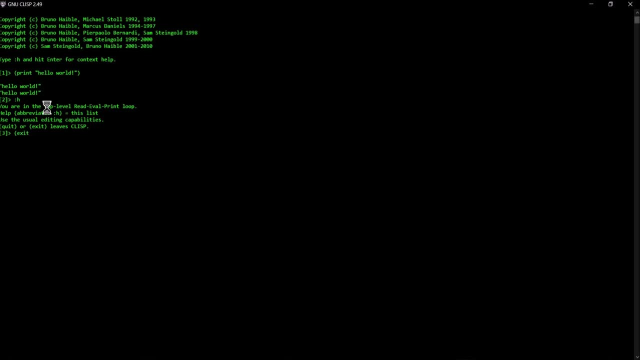 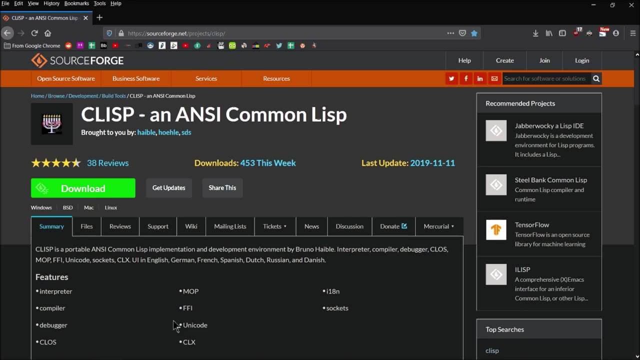 You know, I can call the quit function or exit, Right, And that'll break me out. Okay, So that's one way of doing it. Another way of doing it would be to fire up your favorite text editor, And again, in this video, I'm just trying to get you started. 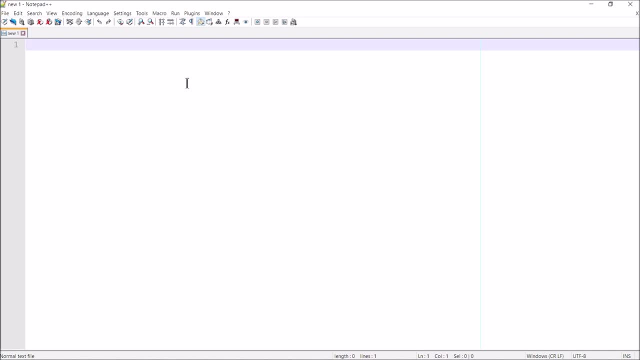 So you can run the program and You know, download it and install it and run, Run some LISP with it, Run some LISP code here. So another way to do it is create your own source code file, And maybe I'll save this on my desktop. as you know, hello dot LISP. 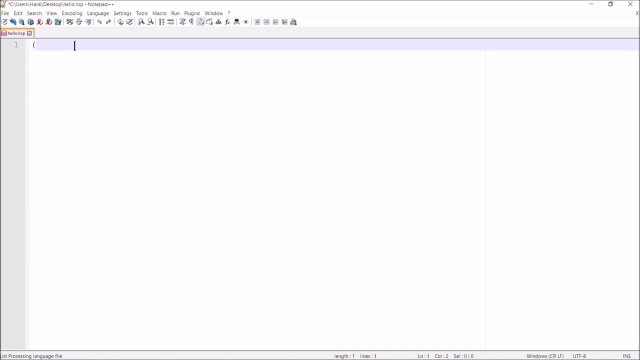 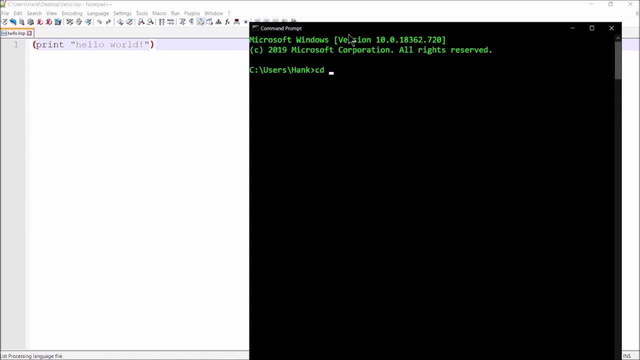 All right. And so then in here you just type in your commands, All right, So print you know. hello world. Done that, Then I can drop down to command line, And I think this is the easier way of doing it. to be honest, 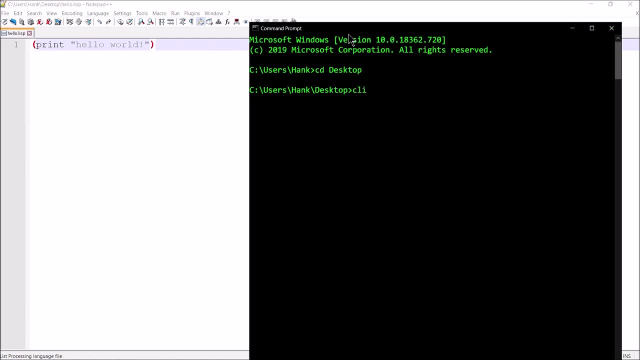 And then you can type the name of the interpreter program And then the name of the file you want as an argument, Right, And then you can see the output. Okay, So I mean that's the basics of it. I mean there's your first little hello world LISP program. 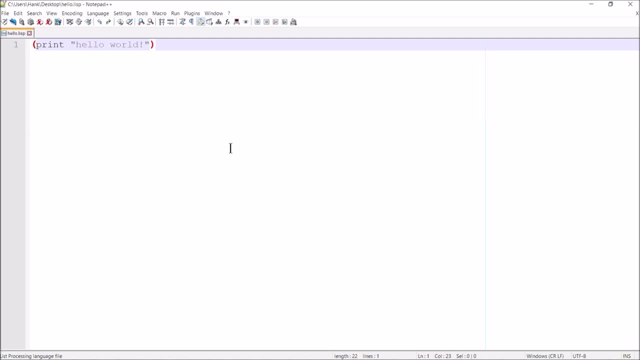 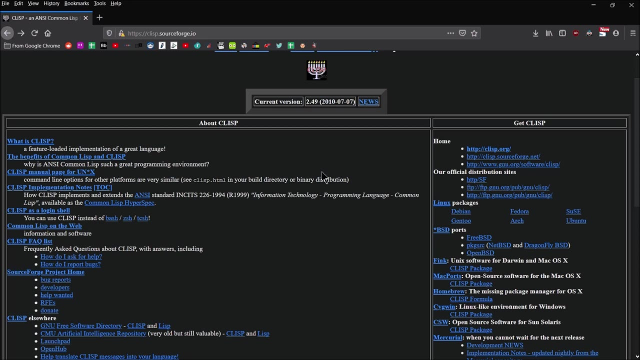 So that should get you started. Okay, So we're back kind of on this landing page for CLISP And you know this is an implementation of the LISP programming language, Common LISP, And if you want to find out more information, get some tutorials and whatnot. 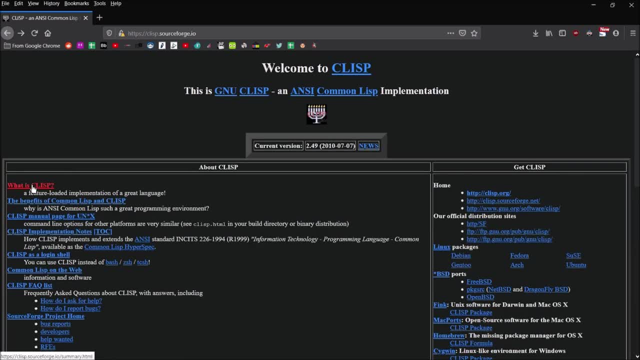 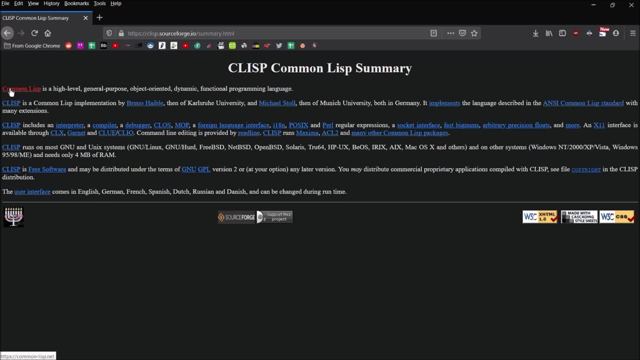 And what you can do is is: you can click on. you know what is CLISP, Right? And then from here there's a link right here: Common LISP. You can click on it. You can click on that. 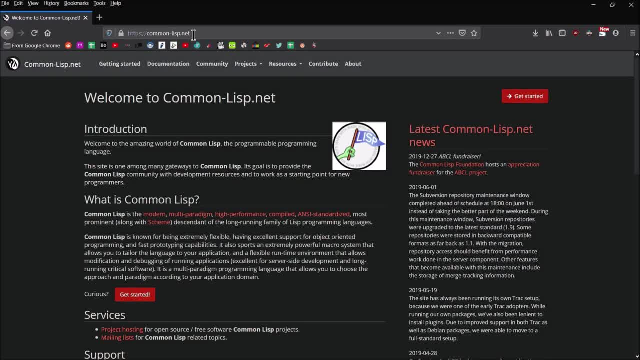 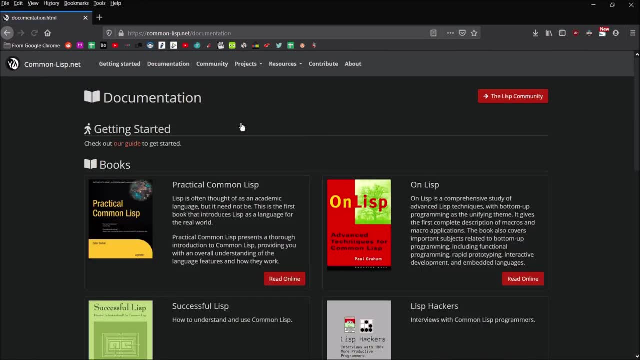 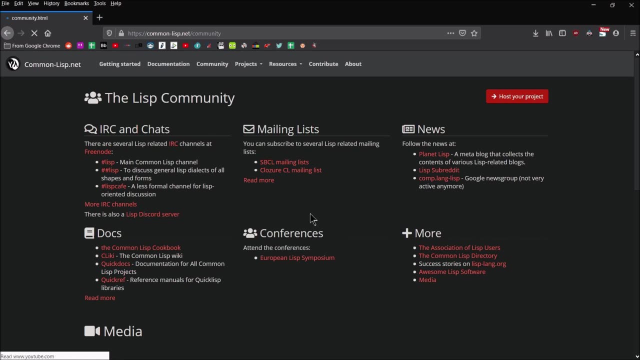 And that takes you to a site called commonlispnet And there's all kinds of information here. You know there's a getting started link, There's a documentation link to different books, A link to the LISP community where you can get on emailing lists, news, IRC, chats, different documentation. 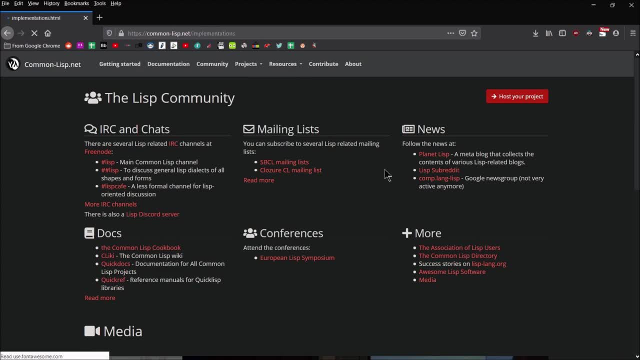 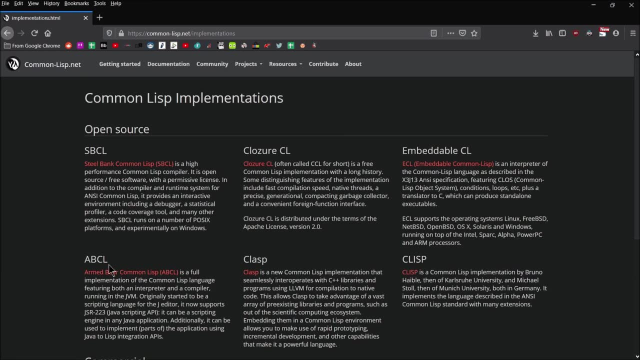 You know, if you want to check out different implementations, You know CLISP was one of them. That was the one that I just did, Right, But there's others too, Right? So you know, pick whichever one you feel comfortable with and experiment. 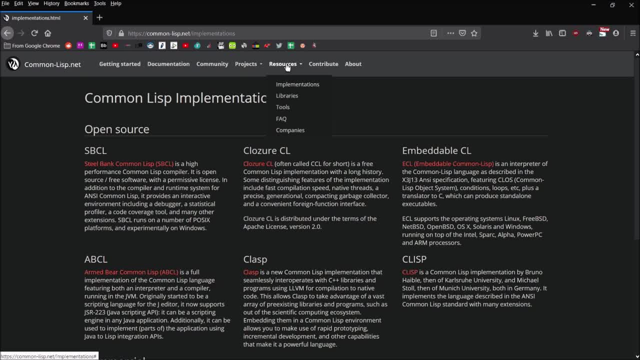 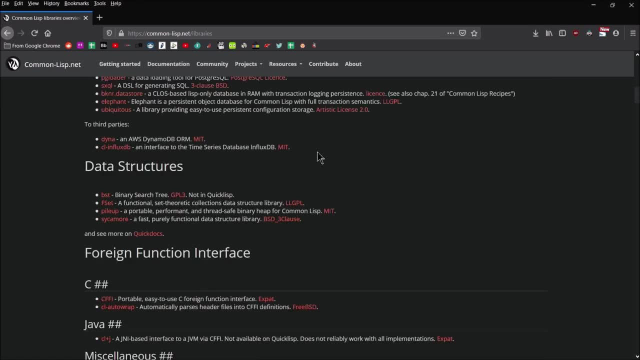 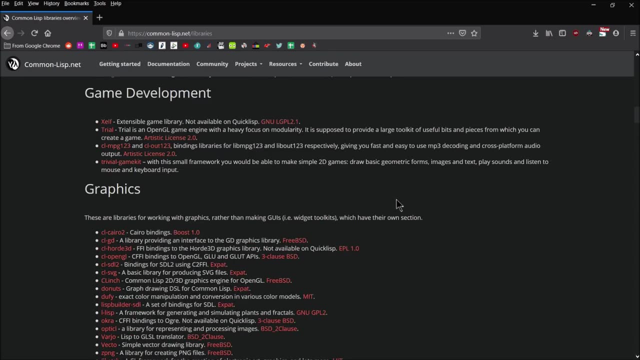 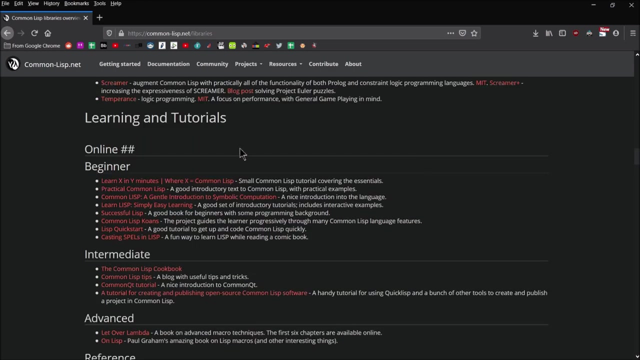 But you can get to additional resources under libraries here And if you scroll down you can find out all kinds of information: Information about GUIs, graphics, game development, You know all kinds of different stuff, Logic, programming. But if you scroll down far enough then you'll get to learning and tutorial section. 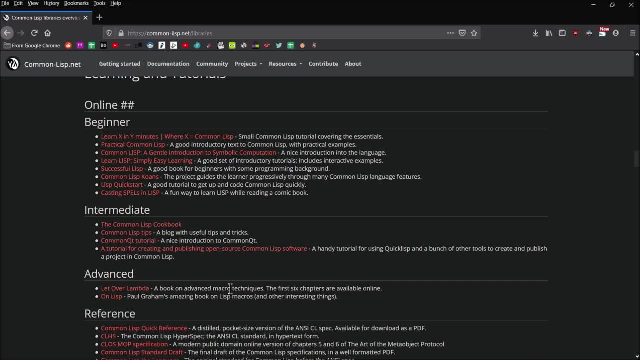 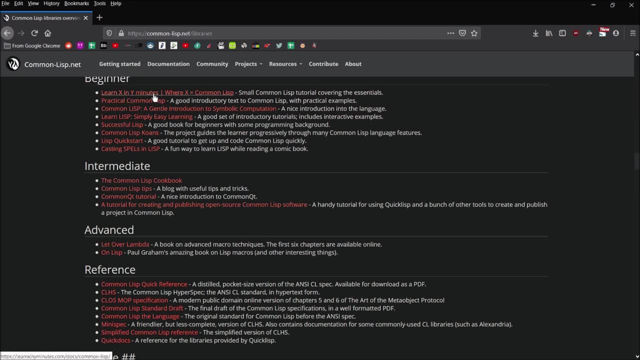 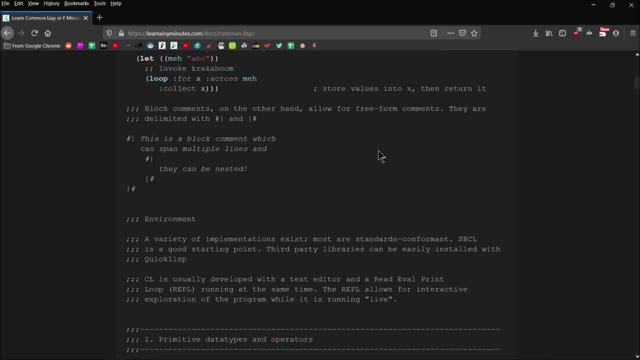 And there's a bunch of links to different free online resources to kind of get you going Right. So here's a couple that I like. I think this first one right here: learn X and Y minutes, Right. This right here kind of just gives you a summary of you know brief introduction. 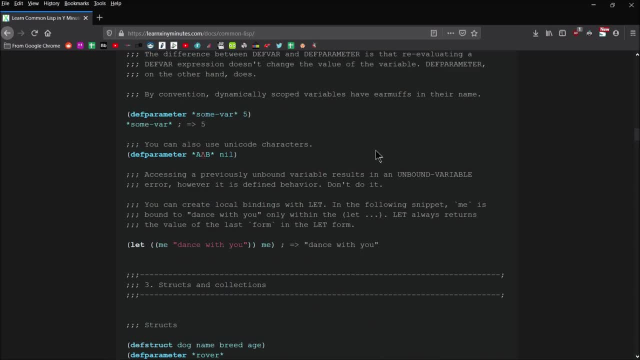 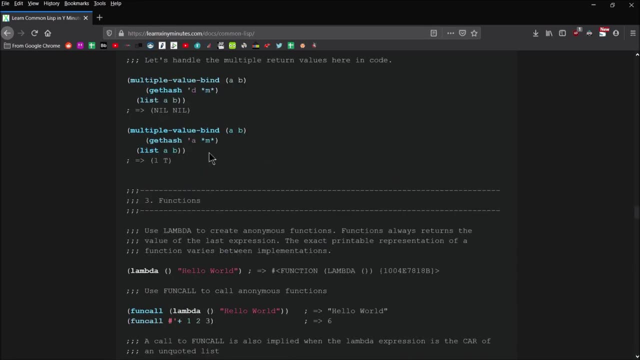 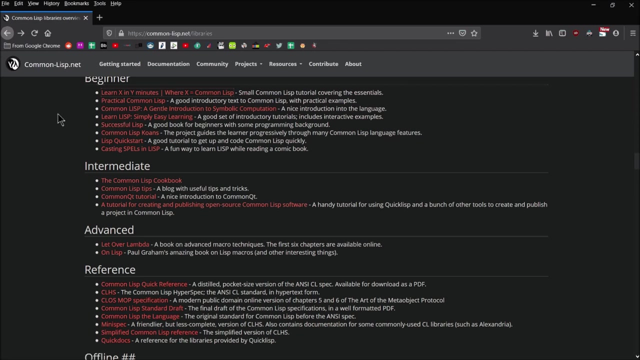 To all the different things you can do in LISP by example. Right, So you can go check this out and get an overview In my class that I teach you know. what I do for my students is I have them take a look at the tutorials point site. 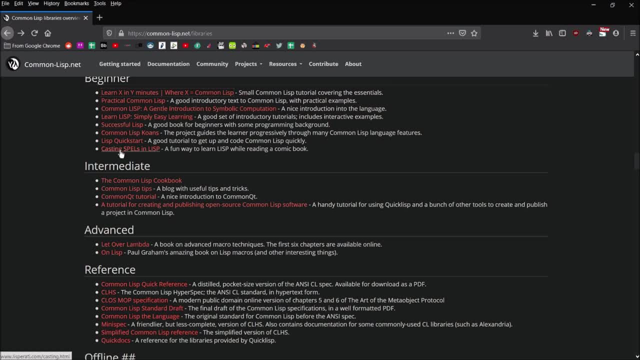 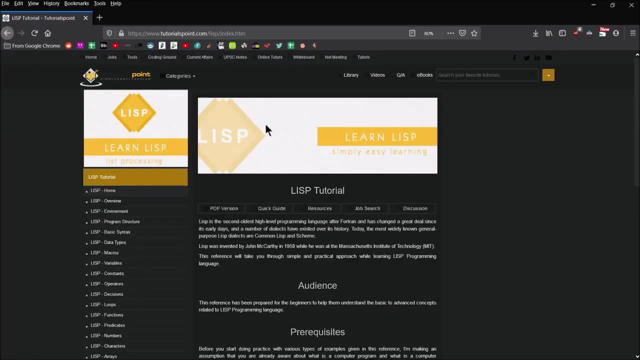 Which is: let's see here. Uh, Let's see Which one. is it Right? There it is Third link. So tutorials, point Um, You know, learn LISP Right. Really simple, easy learning tutorial site. 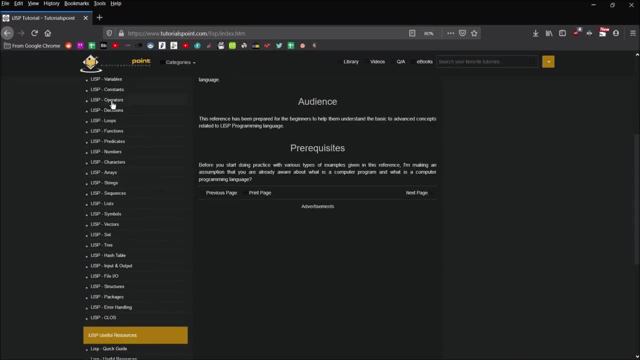 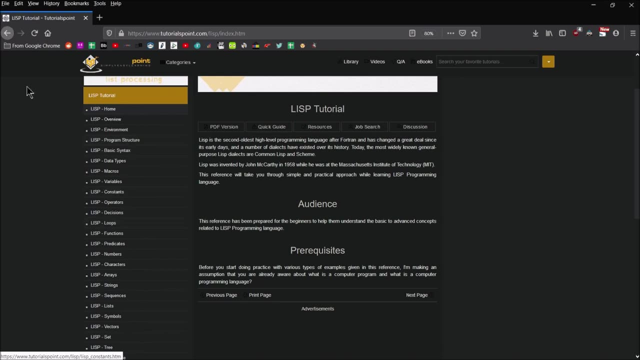 And it's got everything here. you need to really get started Right, Covering all the different topics, All the functionality, Language vectors, Sets, Basic syntax, Macros, Predicates, All that stuff Right. So you know, check those out.